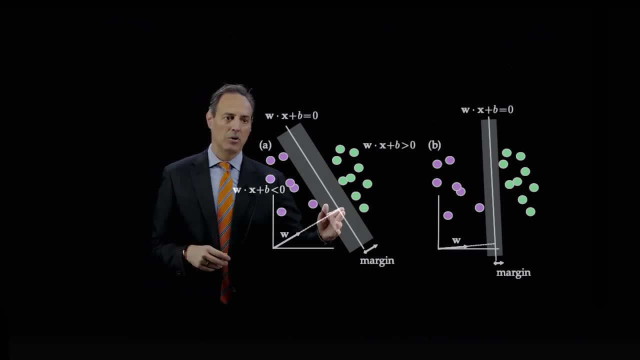 Now, what's interesting about the support vector is this W, which tells me how to get out here to characterize this line, is basically the support vector And in fact, what we want to look at here is: I want to not only find this line, but you see this margin here. I want to penalize everything to keep those balls out of, out of out of this margin. 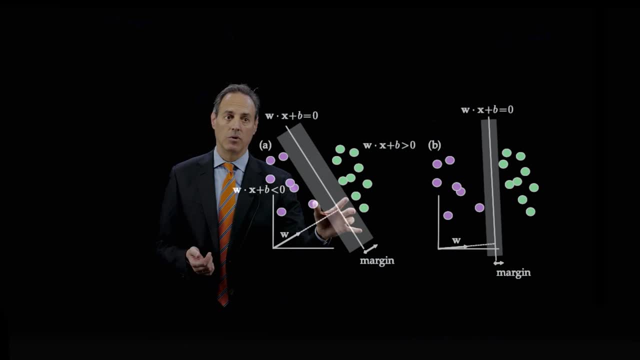 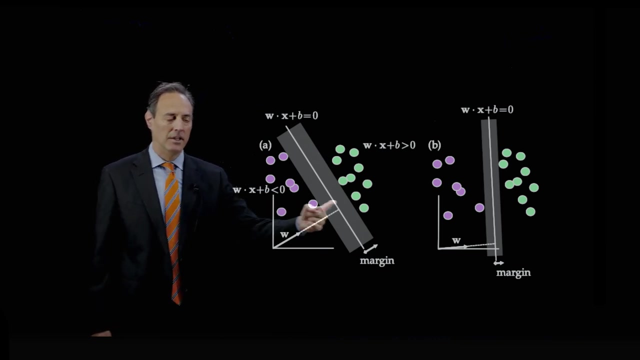 So my goal is to maximize this margin. So in this data, what I'd like to do is figure out how do I construct this line such that my margins are as big as possible. So here is a good representation of the SVM. Here is a poor representation. 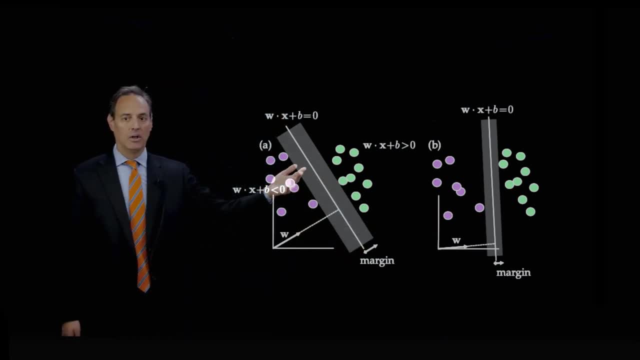 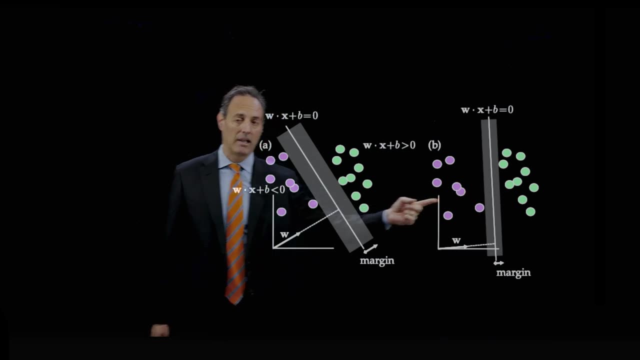 Notice that both of them in training. if this was my real data, would give me perfect separation of the data, right? If you look here, the data is perfectly separated by that line as well as this line, But here the margins. look at the margins. 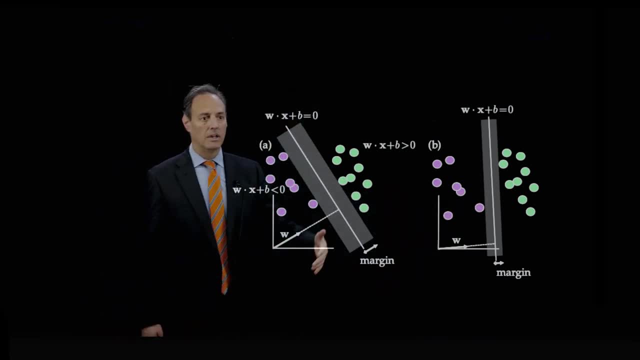 the margin here versus look at the margin there. So my goal is then to find a line, a W vector that will allow me in NB, that will allow me to basically figure out how to optimize that margin. excuse me, Okay, so that is the goal. 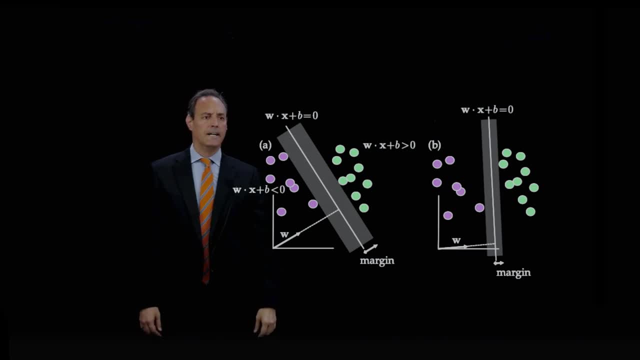 So we're going to go after this and try to train this here and figure out how to set that up as an optimization routine. By the way, notice That the margin has all the balls to the right or to the left of the margin. 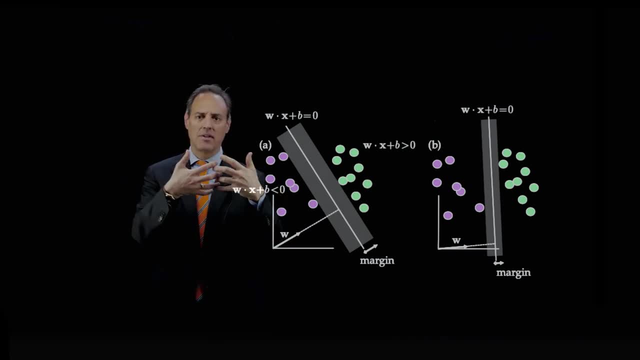 But in practice, you know, we've already seen data where the magenta and green balls overlap on each other's sides. So what you do is you penalize any single ball that is across that line, right? So if obviously you would like to not have any balls from the green on this side, no magenta balls on that side. 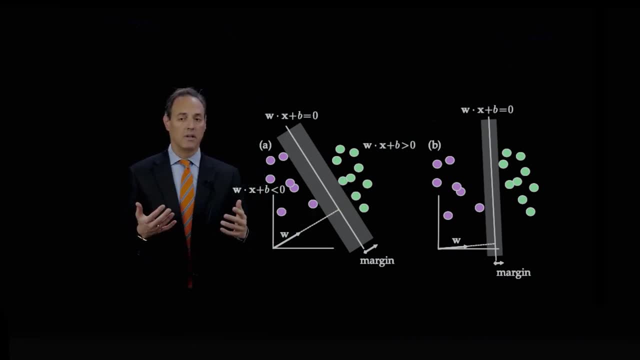 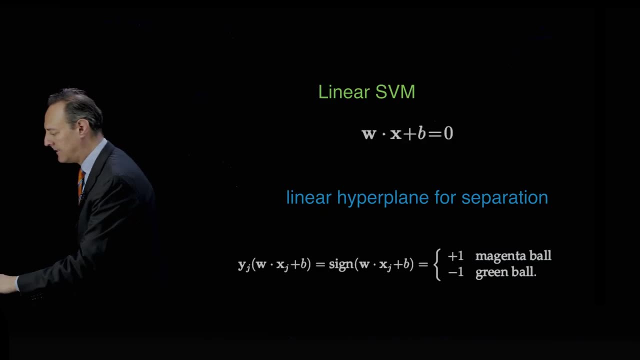 but the penalization that you would impose on the in the optimization would handle that Okay And try to do the best job it can in separating those. So we're going to first start off with this idea of a linear support vector machine. 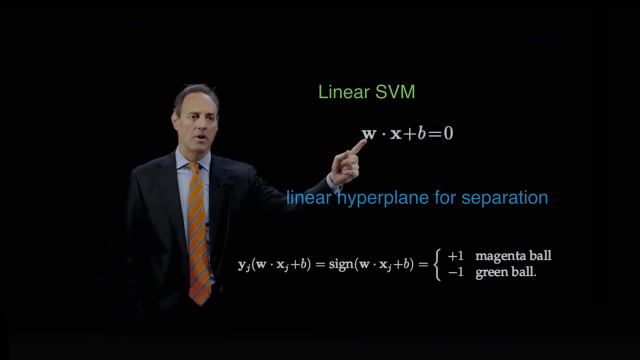 which is exactly what I just showed you, which is say: all right, I'm going to try to find this hyperplane separating the two parts of the data that give me a maximal cushion on each side so I can really maximize that margin. Okay, 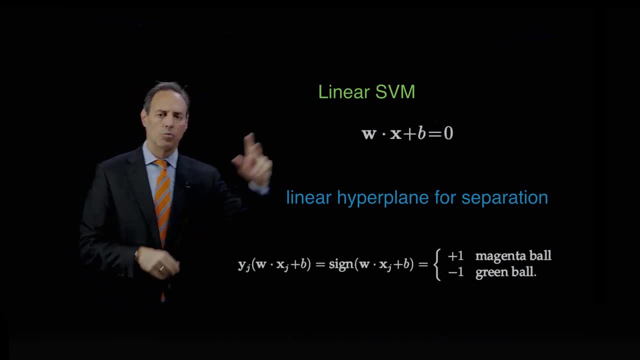 So this is a linear plane of hyperseparation. The important thing that's going to happen here is, once I define this plane, what I'm really going to look at is: then my labels are going to be y, which is a function of wx plus b. 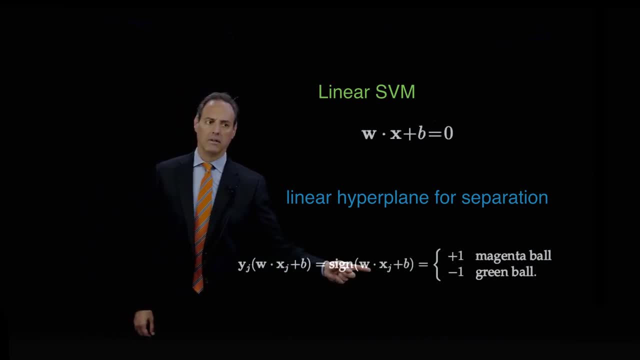 which is actually just the sine of wx plus b. So plus 1 or minus 1.. So I'm just going to take the sine. So if I'm on the hyperplane, this is 0. If I'm on one side it's plus 1.. 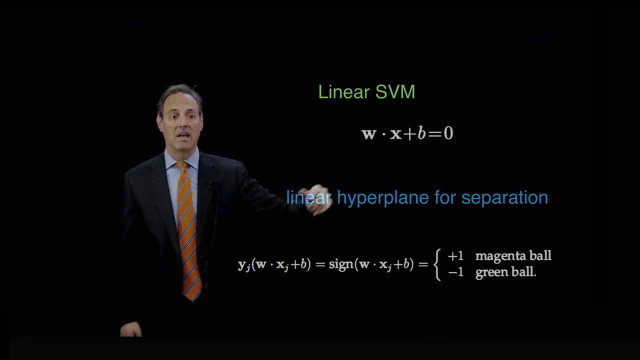 Sorry If this is positive. if I'm on the other side it's negative, and I will just take positive or negatives and make them 1 or minus 1. In other words, the labels of the dogs and the cats. Okay, 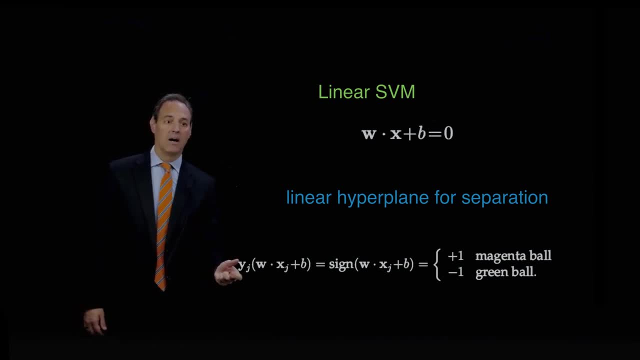 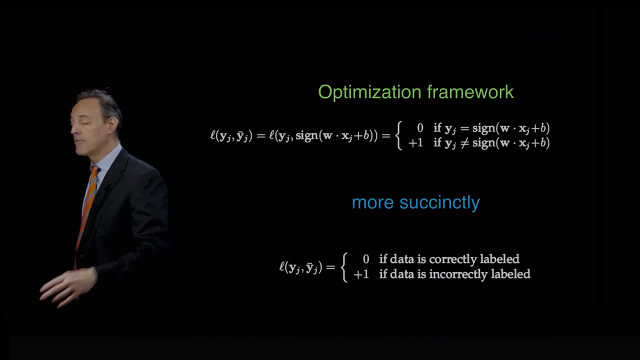 So this is, in fact, my output that comes from knowing my hyperplane. It's an integer plus 1, minus 1, or however you choose to frame your classification. So this leads us to be able to formulate, in fact: 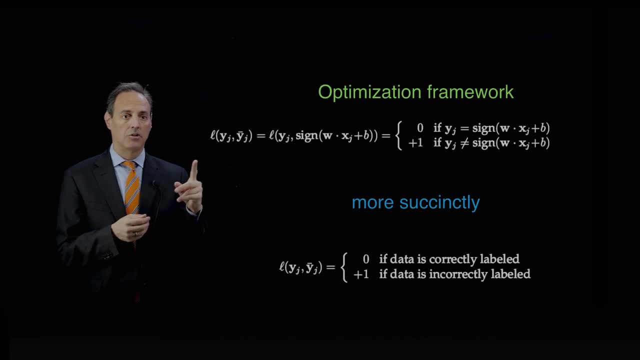 the loss function we need for the optimization procedure. So the loss function is given here and I'm looking at y of j, y, bar of j. So when I train, this y of j is going to be the truth. In other words, I've given you a training data with labels. 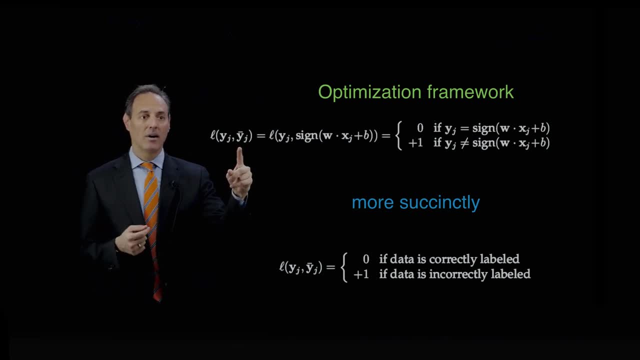 So I know what the y of j's are supposed to be. Y bar of j is my approximation to the label, given my hyperplane, the sine of the hyperplane, which side of that hyperplane I'm on. So this is what I think the label is: y bar. 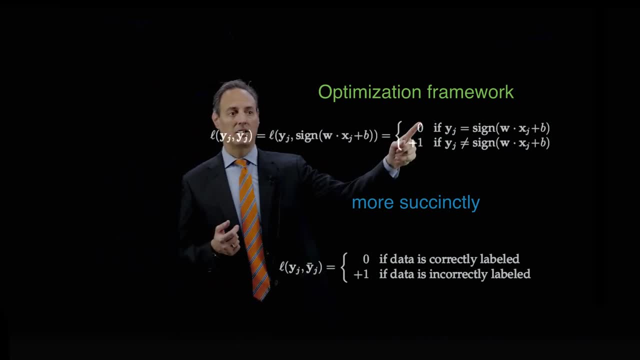 This is what it actually is. So this thing is actually 0 if in fact I got it right, and plus 1 if I got it wrong. So, in other words, this is a more succinct way to say this- This loss function is 0. 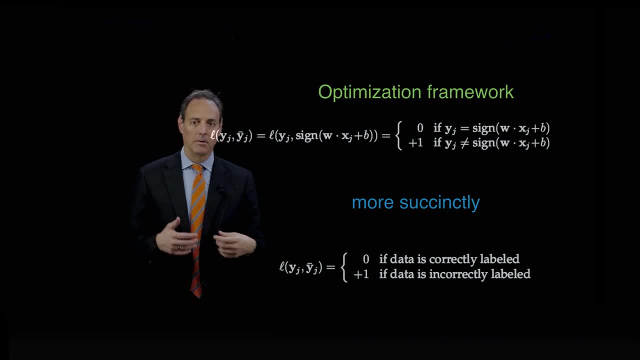 If you labeled a piece of data correctly, it's plus 1 if you labeled it incorrectly. So obviously, everything you get wrong you hit a penalty of plus 1.. Okay, And of course, the more you hit wrong, the higher your losses are going to be. 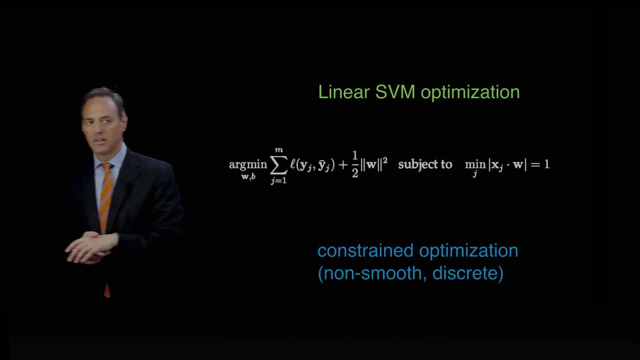 So we want to basically minimize over those losses- and here is the linear SVM optimization model that you can write down for this. Minimize this loss function with the norm of that w vector as well, so you also make this as small as possible if you can. 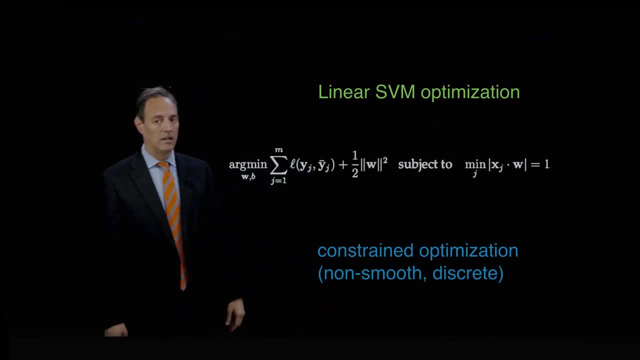 subject to a constraint. Okay On the. So this is, You have to minimize, So sorry, x of j. w is 1, length 1.. Okay, So this thing here is your basic formulation of the support vector: machine optimization. 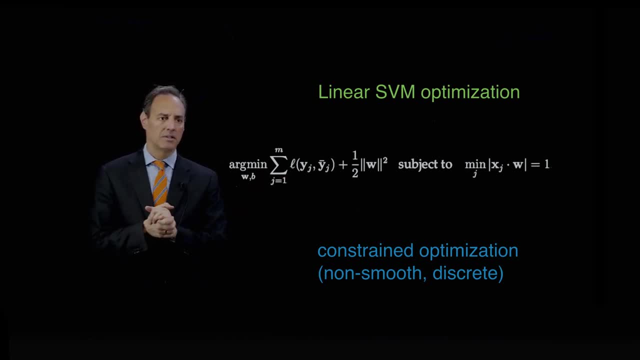 So it's a constrained optimization. You want to minimize the loss function, and one of the difficulties in the loss function- especially if you go to high-dimensional data- is oftentimes the way you would solve a problem like this is through, maybe, gradient descent. 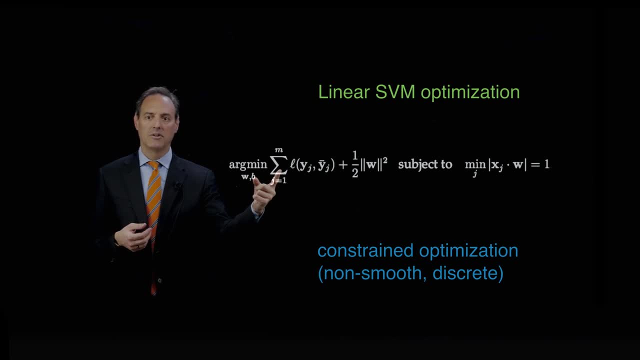 but the problem is this loss function is discrete and non-smooth. right because it's you that take a 1-penal loss function and it's not a penalty or a 0, so it's As you walk through. it's very hard to produce gradients on non-smooth functions. 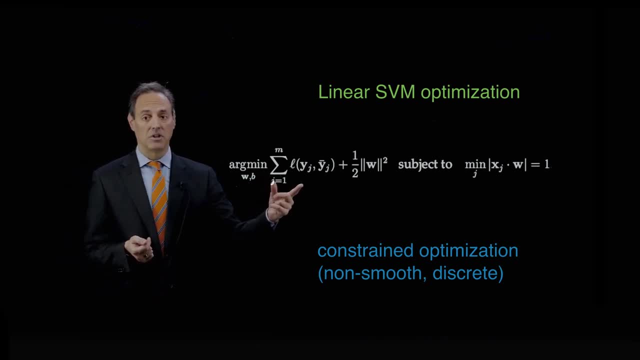 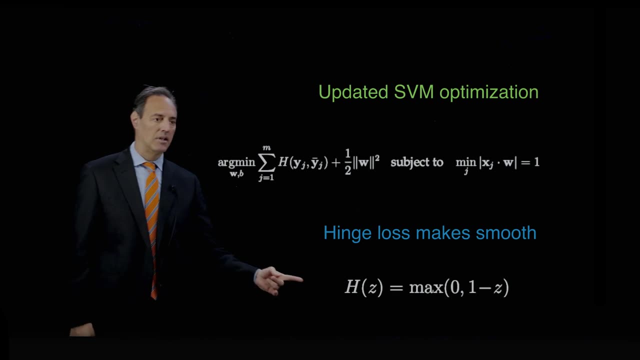 So oftentimes. this is not the way that the optimization procedure is actually solved. It's actually solved by introducing what's called a hinge loss. Now, the hinge loss is given here. so what you're doing essentially is smoothing that loss function. 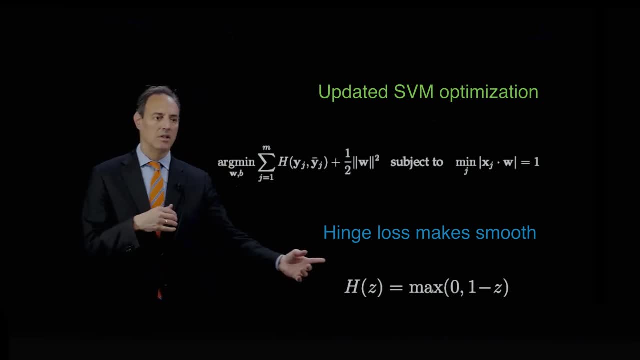 Instead of being 0,, 1, and taking these discrete jumps. it will let you smooth this out so that, if you apply gradient descent on here, you have a smooth function and, in fact, an easy one to differentiate, which is exactly what you like. 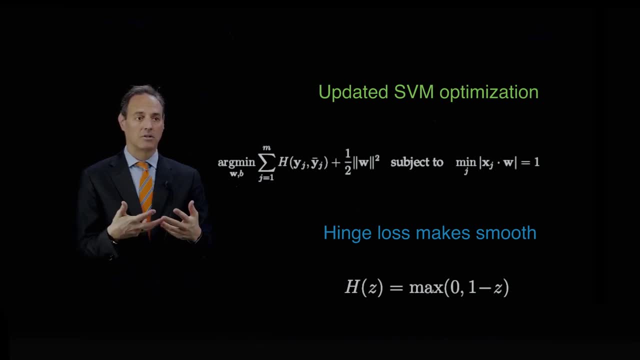 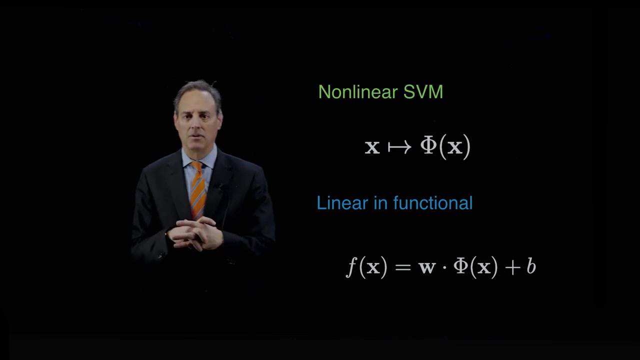 So this is, in fact, the SVM type of architecture for finding, optimizing to find that hyperplane that best separates the data. But that's not what makes SVM special. What makes SVM special is this ability that people learned early on is to say, like well, I don't have to, in fact, work with just the data x. 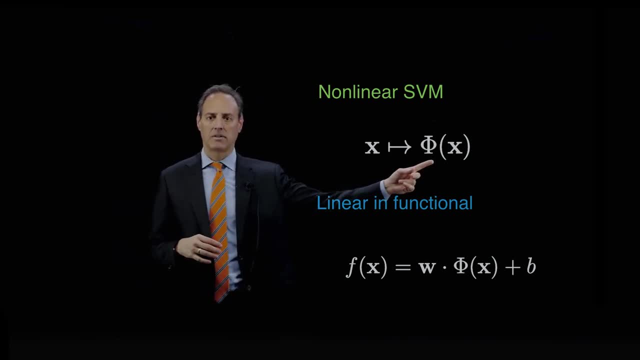 I can, in fact, work with some functions of x, In other words, I can create functionals of x. In other words, I can take this into higher dimensional representation space through this phi here, which takes me not, doesn't force me- to live in a linear space. 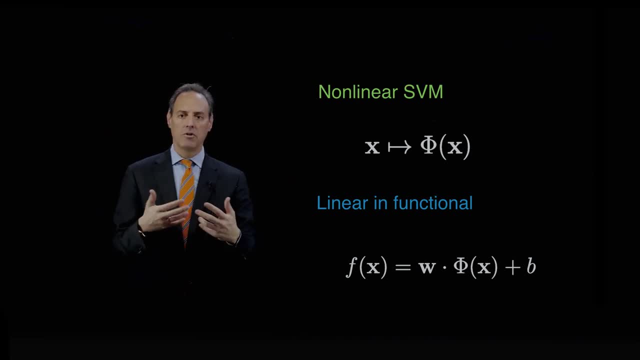 I can lift it into higher spaces, other versions of the variables- And I'm going to show you concrete examples of this in a minute- But what this allows you to do is if I can move into an alternative representation which is much richer, much higher dimensional. 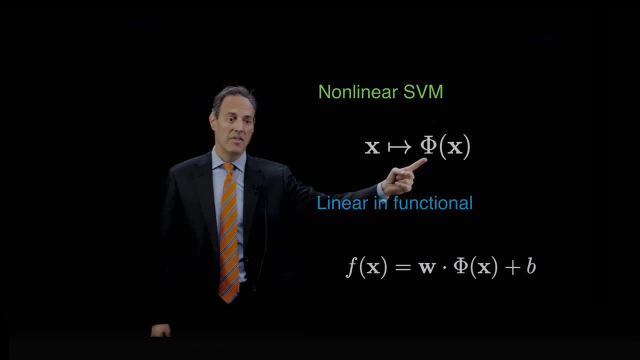 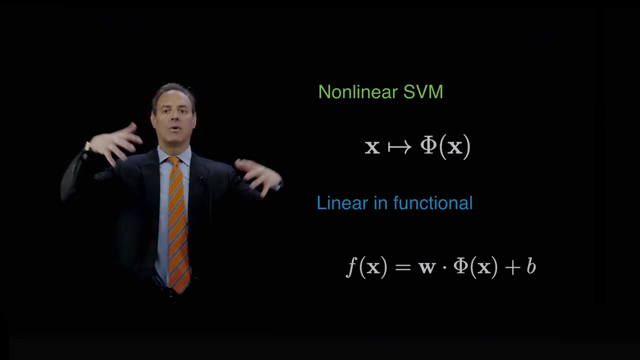 in other words project into higher dimensional space. then I do my linear functional here, in other words my hyperplane separation in this new variable. So the goal of SVM is to take this, take all your data into a higher dimensional representational space. 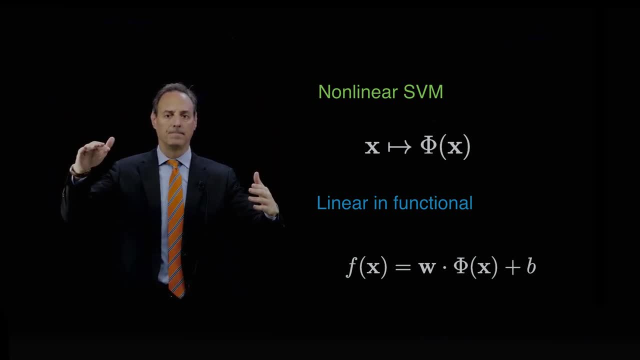 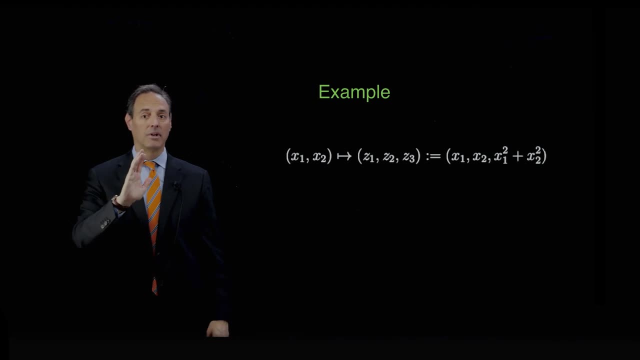 and then draw hyperplanes separating the data. Okay, So let me just show you here This is going to. I'm going to give you one example that's going to hopefully highlight this to you. I have data x1, x2.. 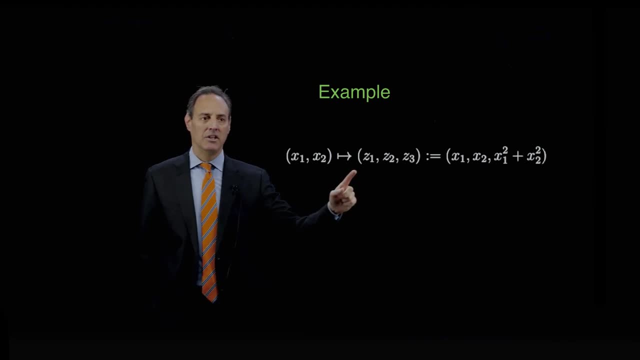 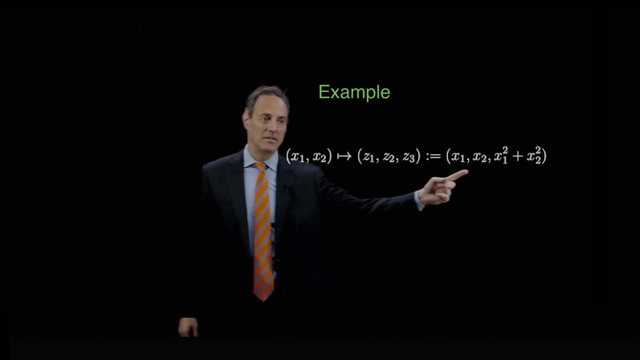 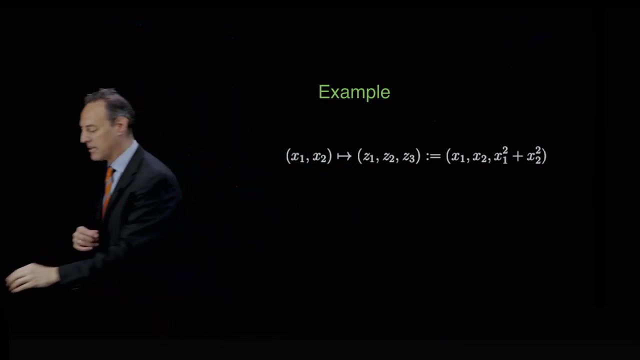 From that data I'm going to move into a new space: z1, z2, z3.. So I went from two dimensions to three, And the third dimension I define as x1 squared plus x2 squared. Okay, So I went from two dimensional data to three dimensional data. 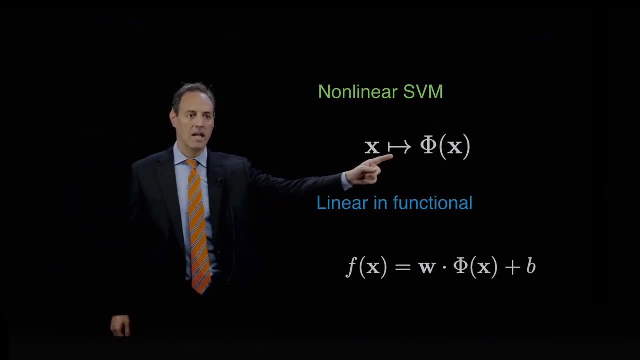 So, just to go back, this is just this process right here, And I can define projections into all kinds of directions with this, And this is exactly what I want to do, because most data isn't easily separated with a line. However, if I go to higher dimensional spaces, 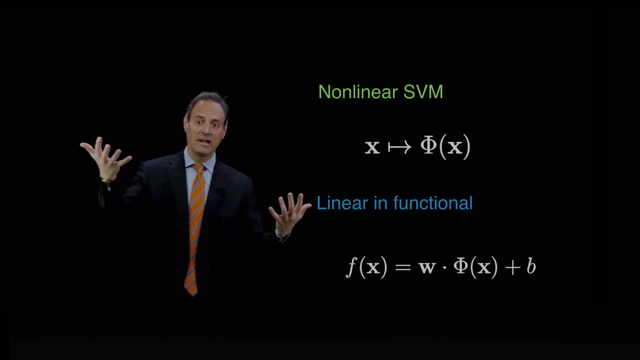 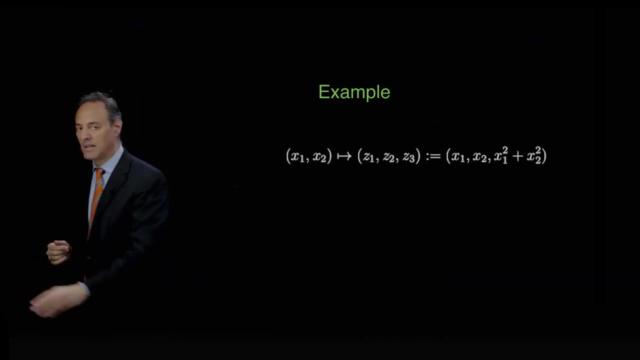 I'm going to show you in a moment. all of a sudden lines separate data amazingly well, or hyperplanes do Okay. So the goal is to project to higher dimensional spaces where hyperplanes can very easily separate your data and give you very good margins between the different clusters. 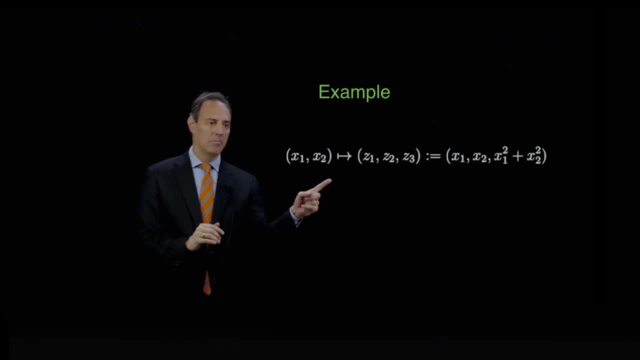 Okay, That's the goal. So here I'm going to give you this example. I've gone from x1, x2, from x to z. What does that buy you? Well, let me give you a really challenging data set. 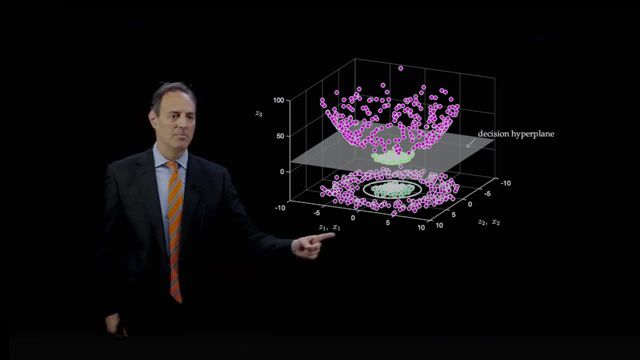 which is trivial now with support factor machines. Here's my original data in the x1, x2 plane. So I have the magenta balls down here and the green balls on the interior, So notice the optimal separation between these. would be sort of this circle here, right? 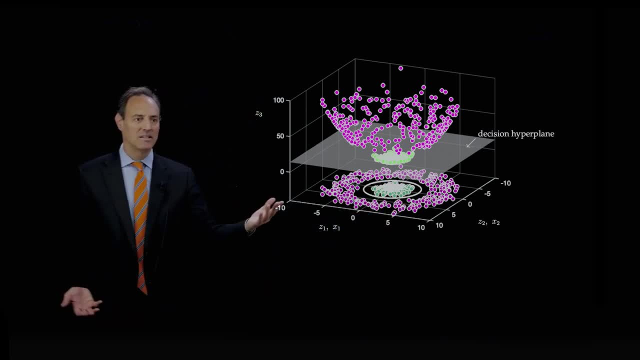 And, of course, when you do these linear hyperplane lines, they're not circles, they're lines, And there's no easy way to separate the data with a line. However, if I now move to the new variable set z1,, z2, z3,. 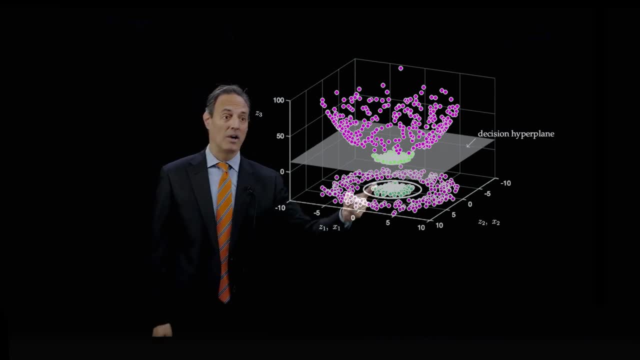 where the z3 direction is x1 squared plus x2 squared. this is what the data looks like up here. I have the magenta balls sitting above the green balls And now I can very easily draw a hyperplane separating those magenta from the green. 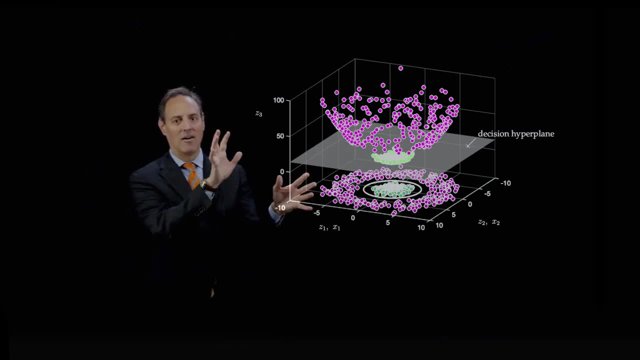 Okay, So this is a canonical picture of what going to higher dimension can buy you in terms of being able to do discrimination and classification tasks, And this is why SVM has become so popular is because data lifted into high dimensions, you can use linear discriminators very effectively. 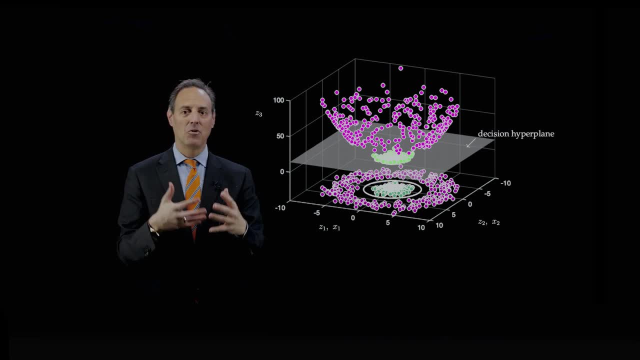 The cost of this is that if you have high dimensional data, then you're even going to go to even higher dimensional representation. So it's very costly to do SVM in many applications, Partly because what you're doing is going to be doing from already a high dimensional state space. 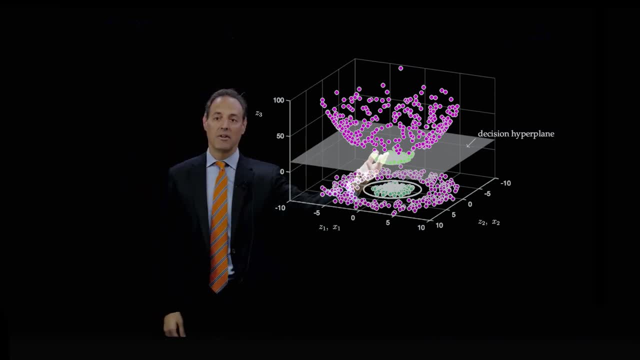 to just continuing to go even higher dimensionals by making up these other variable directions. Okay, So that's an important feature, but you can see how powerful it is if you can do it. There's one other interesting thing that happened with SVM. 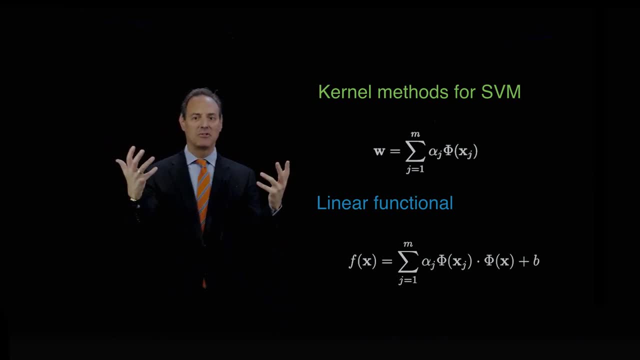 which is by committing to going to very high dimensional spaces. you get yourself into a very large computational optimization procedure, And oftentimes this may be, in fact, intractable. However, one of the things that was realized early on is what are called kernel methods for support vector machines. 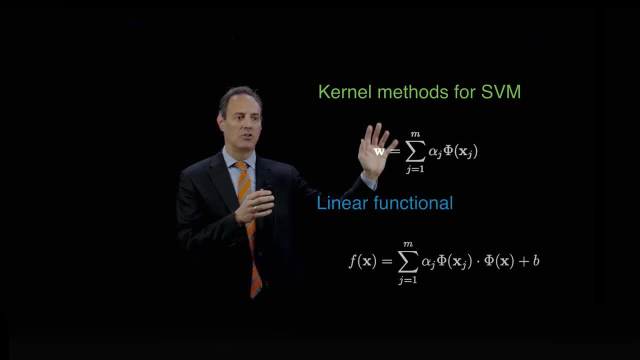 And this is this idea- that if I start projecting into these planes- so this is just generic representation to these functionals- then what I can do is say I'm going to take this W and I'm going to project it into these spaces. then my functional here is going to be: 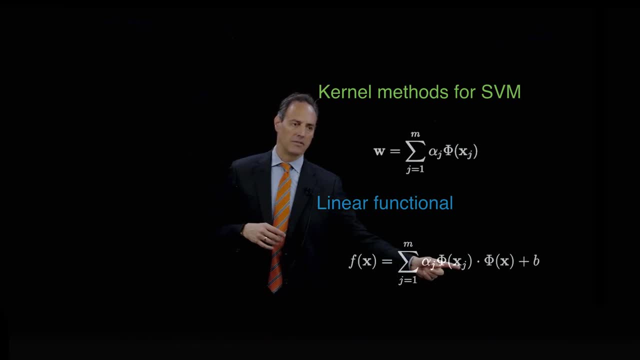 the sum of these alpha j's, alpha phi of x of j, Dotted with phi of x plus b. So what I have to compute here, when I go to very high dimensions, is this dot product between all of these high dimensional representations of the data. 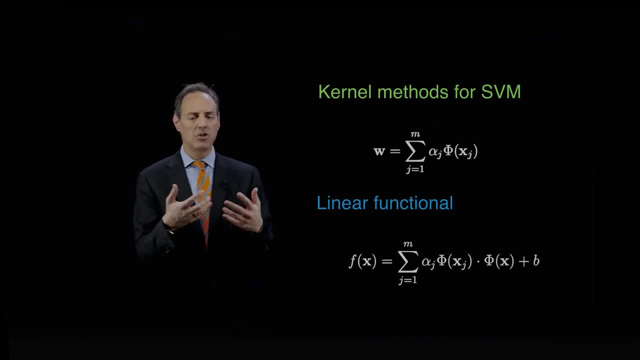 But what people realize in kernel methods is say: why don't, since I'm doing this, why don't? in fact, I just define that as some kind of kernel, In other words the idea being say, I will take this guy and I'll say, since I have to produce this, 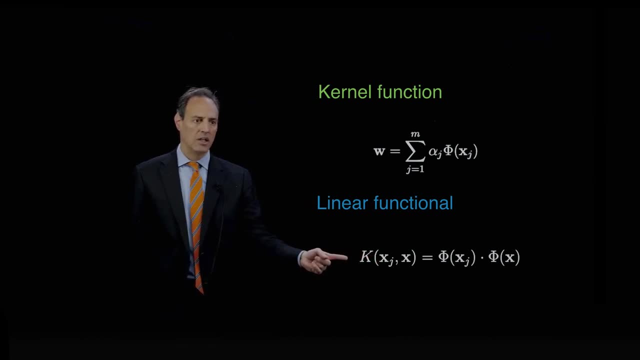 I will reproduce this as what's called a kernel function. In other words, this is the thing that's killing me to compute, because I'm projecting everything into very high dimensional spaces and I'm having to dot product them together. So instead I'm going to represent that kernel in a much more compact way. 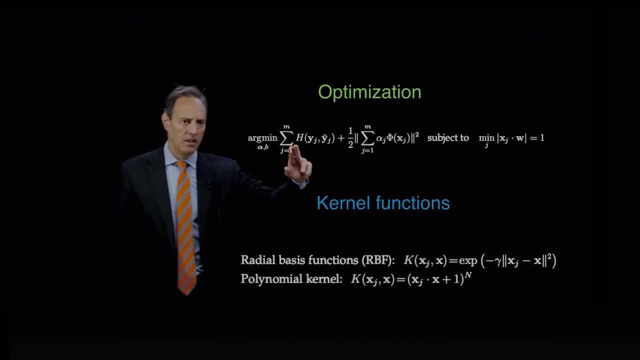 Okay, First of all, by the way, here is now the representation of this thing, which is some hinge loss with these functionals that you want to put up here. So the optimization procedure hasn't changed much, but it's now being done on a much more complex. 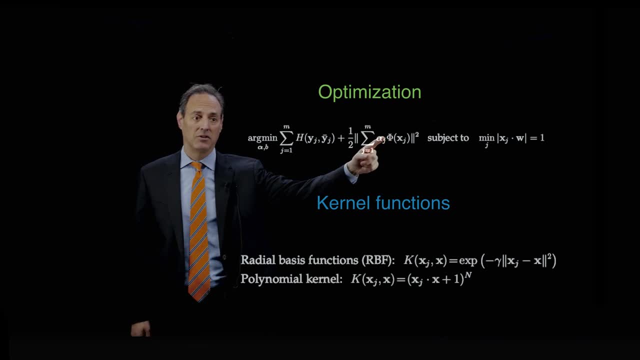 and much bigger scale, because you have all of these functions you're projecting to. But now what you do? you say my kernel function. let me assume it takes on very simple forms. In fact, for instance, the kernel here could be something like a radial basis function. 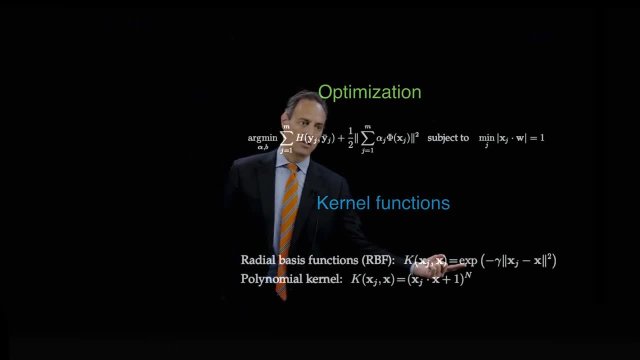 where all you're doing now is producing this exponential Gaussian between data points or polynomial kernels. So this is a very compact representation of this thing here, which is typically expanding into a very large space. So what you often can do is say: well, this often can look like a Taylor series. 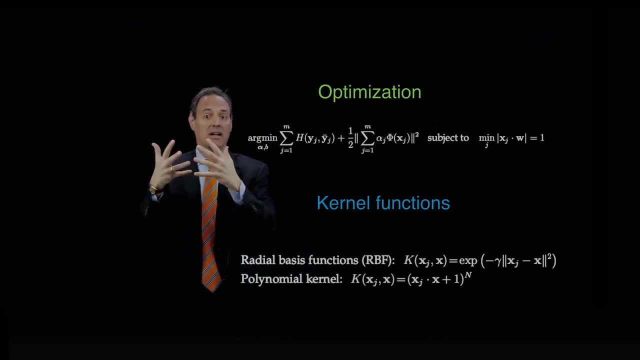 and Taylor series can often be very compactly represented, for instance by exponentials sines cosines, So you do that here instead. So this is a compact way of representing a very high dimensional projection into the space. but the compact representation gives you a very tractable way to compute this. 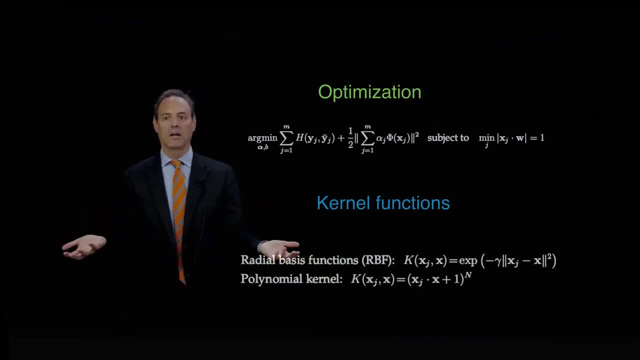 So these kernels become really important. It's called the kernel trick because now I just got around having to do a really expensive optimization by choosing some kernel. that effectively projects me into an exceptionally high space, but I can compute it very easily on the data. 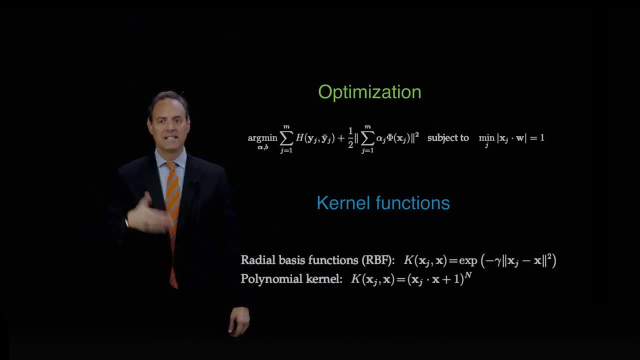 So that was a really important step forward in the optimization procedure for the SVM. because the SVM is, in fact, highly successful because when you take data and you project to high dimensions- as the example showed- you can very easily now draw hyperplanes between the data. 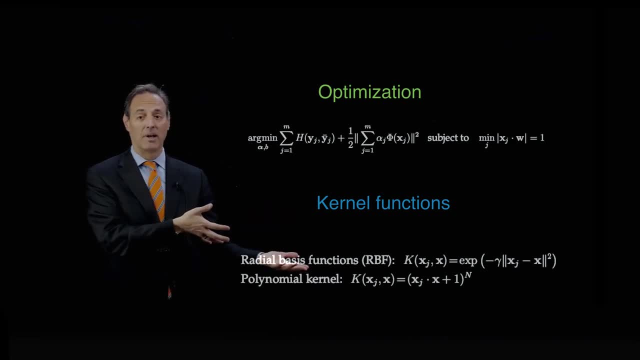 and do a pretty good job with it. You just need a tractable way to go to scale with it, and the kernel method does that. There's a lot of more details about the optimization procedures and innovations on this. This is more just to highlight some of the key themes that go along with SVM. 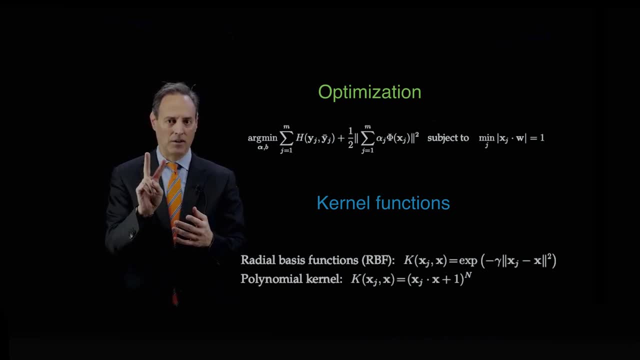 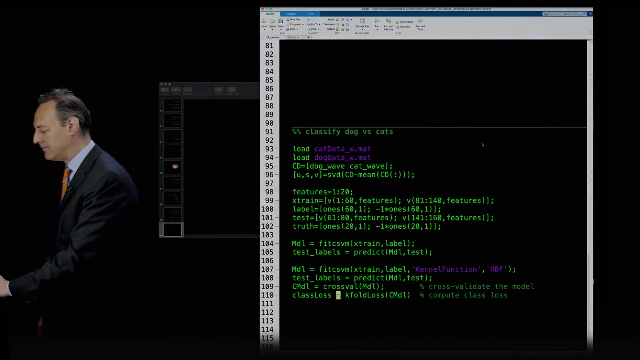 And just to bring it back, two key things: Project to higher dimensional spaces, make up some functional representation into higher dimensional spaces where linear discriminants work. And number two: do something like a kernel trick to make that a tractable process. Okay, so let me just show you how to run an SVM inside of MATLAB. 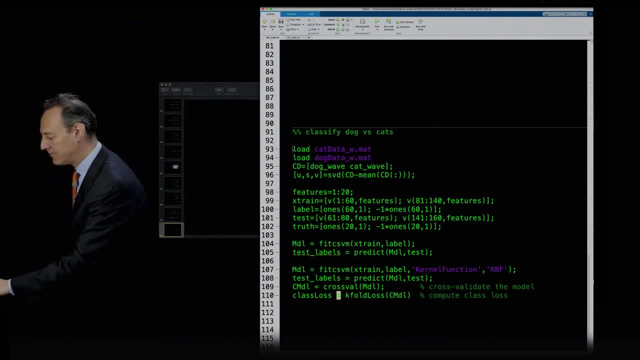 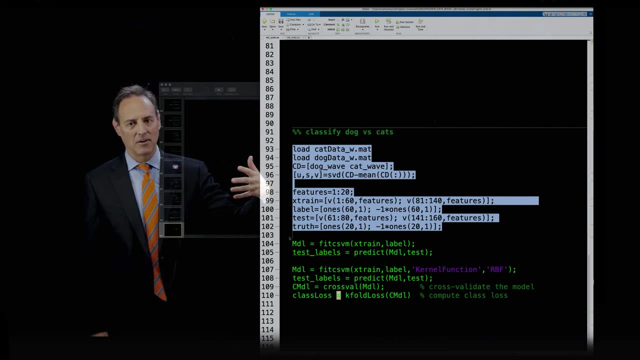 Here's the code. So all I'm doing up here is loading the cat-dog data. We've been playing around this for a long time. In the last lecture I took the dog-cat data and showed how to do this with linear discriminants. 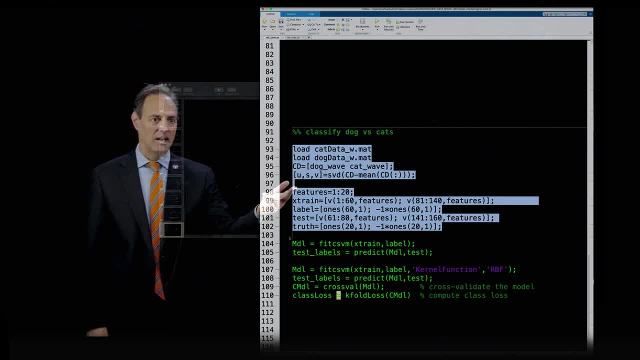 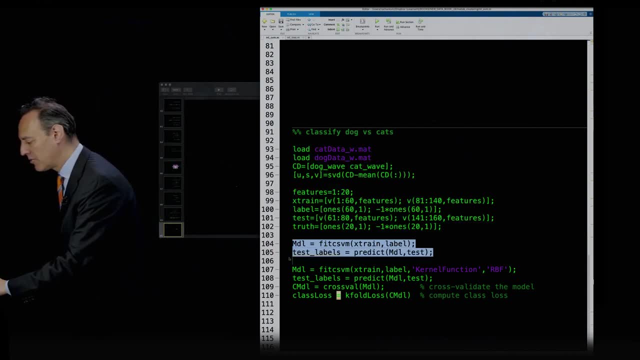 but now I'm going to do it with SVM. So load the cat-dog data, stack it up, pull out the features and the labels and now let's run an SVM on it. So this should be fairly standard by now, And here's what we do. 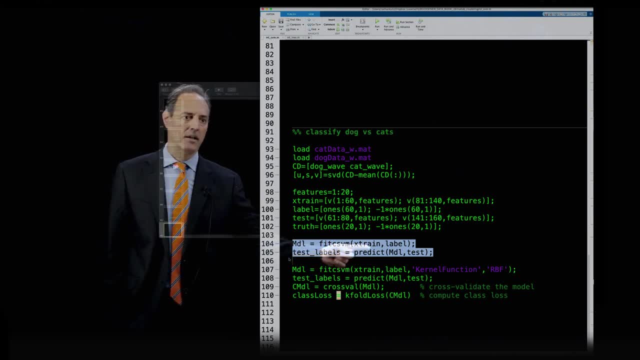 Fit- see SVM- training data and labels- And it's going to give you back this thing. object: model MDL. Okay, so I'm going to go fit the data. All I have to give it is training data, which is the actual data plus labels. 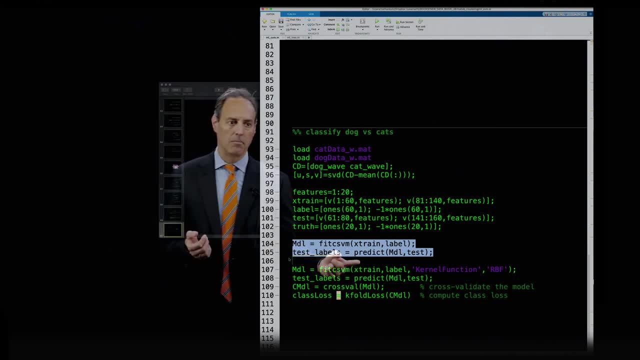 It's going to build a model And then, if I want to see how well it works, I can use the predict command: Predict on the model. Now I can run the test set through and it's giving me the test labels. That's it. 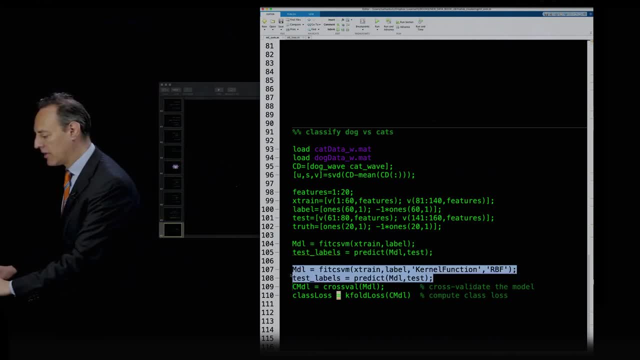 Okay, And if you want to use one of the kernel tricks on this thing, all you've got to do is fit SVM. Here's an option: Kernel function, RBF, radio basis function. So you can pick different basis functions there as you wish. 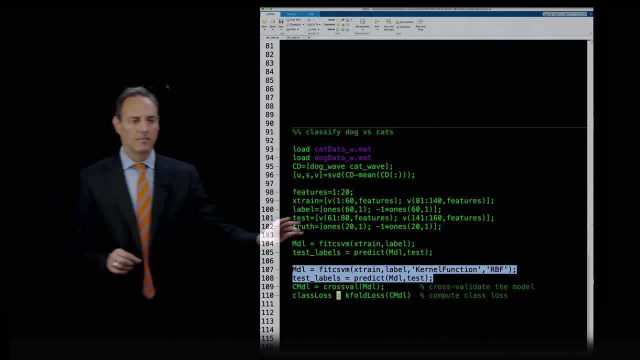 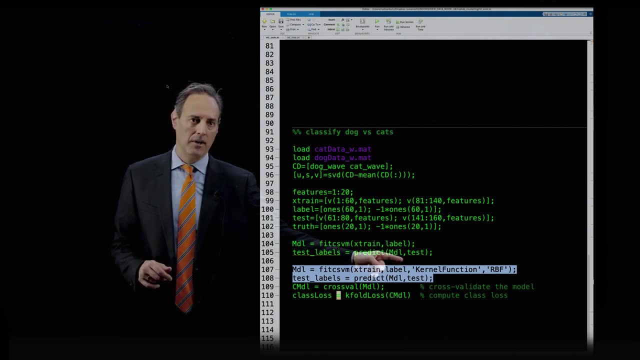 So this is a very powerful algorithm that's available to you and allows you very quick access to kernel methods as well. There they are, And so you have this ability to just very simply train on one of these very high-end methods, And what this is doing again is projecting into high-dimensional spaces. 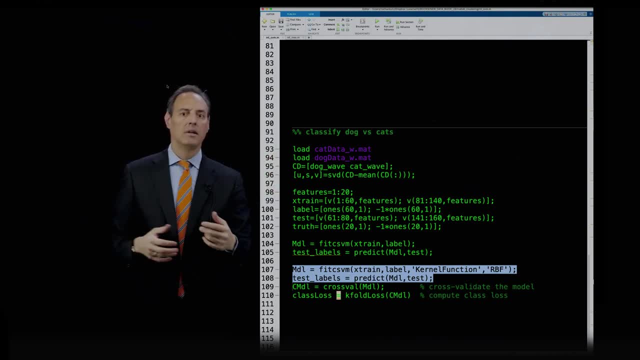 trying to build linear classification lines, And so when you give it a test data set, it's going to also project into these higher-dimensional spaces. You've built all these linear classifiers, or linear hyperplanes up there to separate the data, and it will give you back your results. 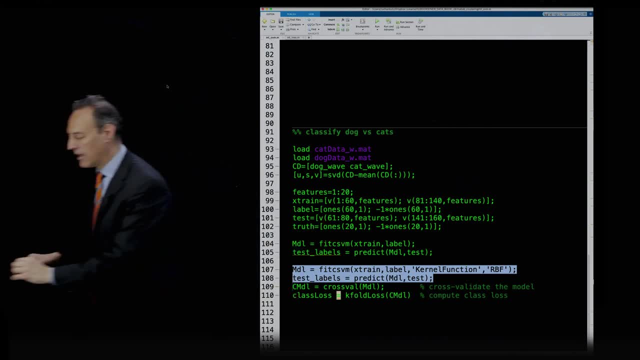 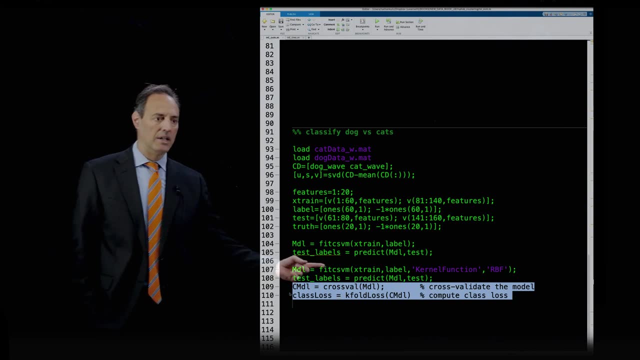 Okay, You can even get very nice diagnostics out of this. So this model structure cross-val MDL so it can cross-valuate the model, give you a cross-validation statistics as well as k-fold loss, which gives you the class loss across things here. 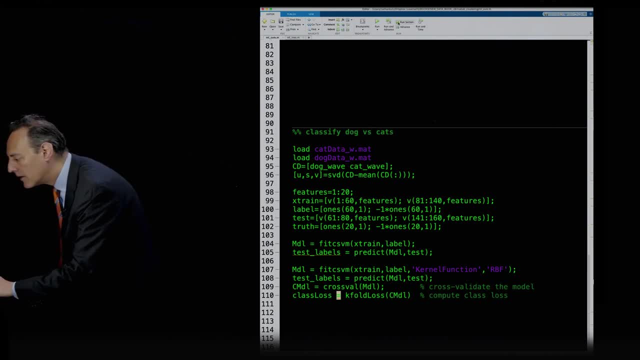 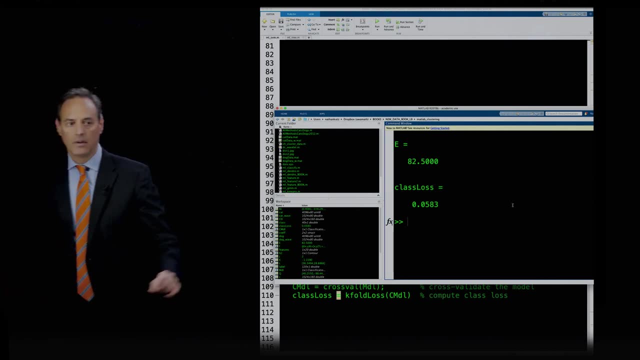 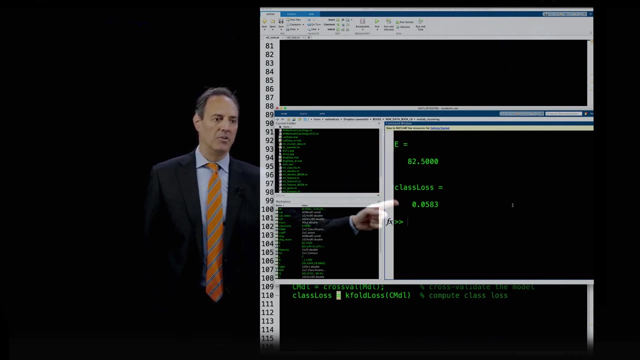 So let's just run this piece of code here And there it is Okay. So the class loss: here it is 5%. So, by the way, I think that was from a previous run we had done, But that's what comes out of this. 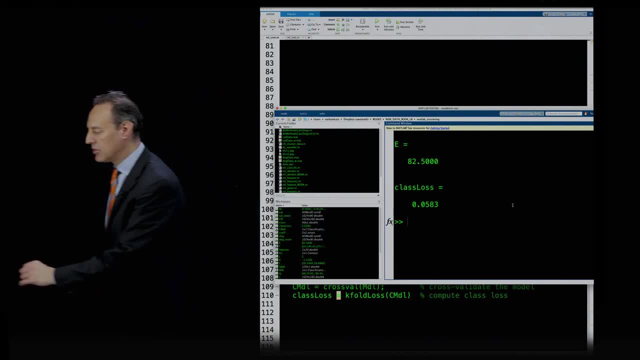 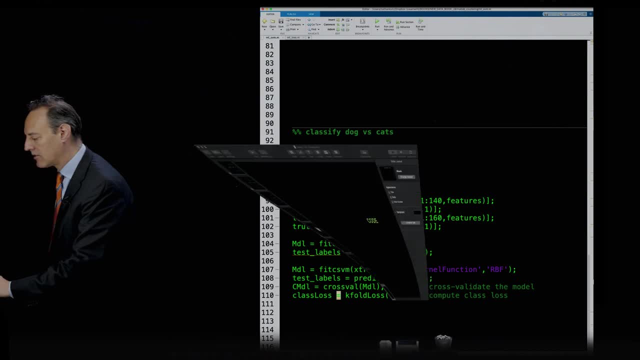 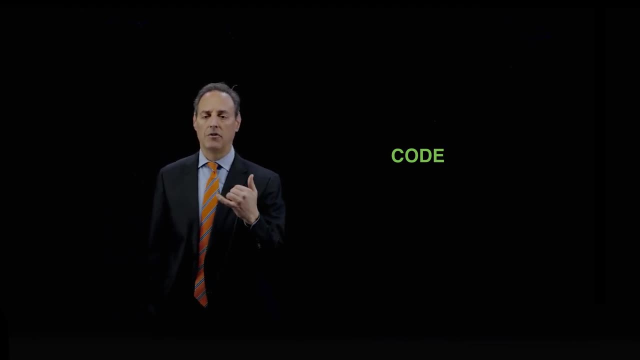 Of this class loss from there. So lots of good features and diagnostics out of the code and it's very simple to execute. Now you have the power of an SVM engine at your fingertips- And, by the way, Python has something similar- and you should just have in mind that if you're going to use supervised algorithms,